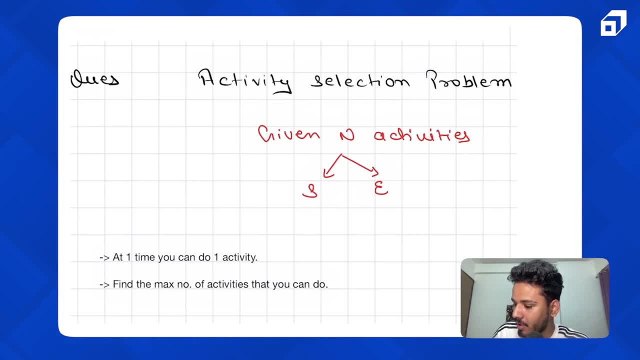 So question is very simple. You are given some activities. What do I mean by activity? You are given start and end time of an activity. okay, At one time you can do one activity and you have to find the maximum number of activities that you can do. 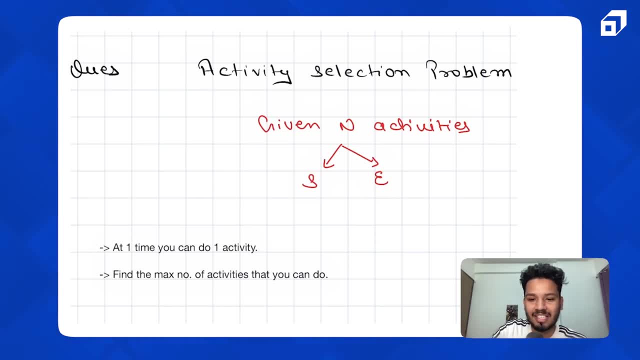 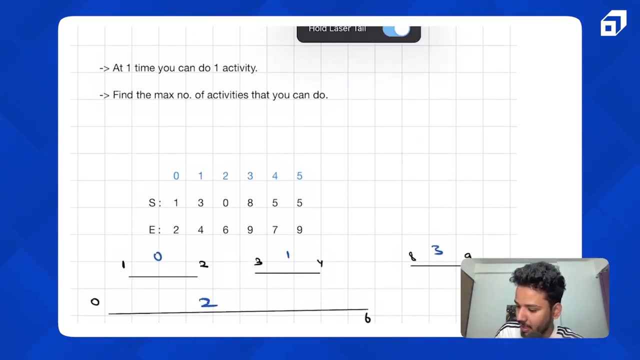 So what's the best way to understand anything? via an example, right? So let's just take an example. So say this is the array given to me: Start array and end array. So first activity or 0th activity starts at time 1 and set time 2.. 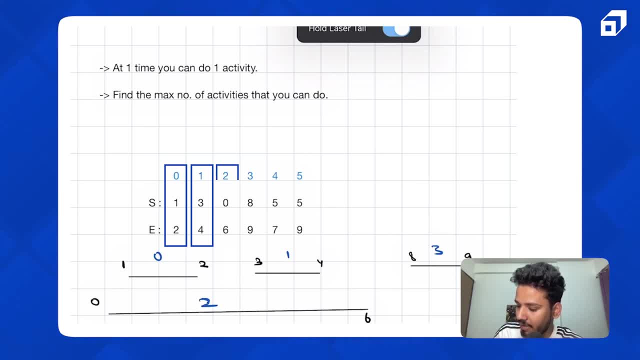 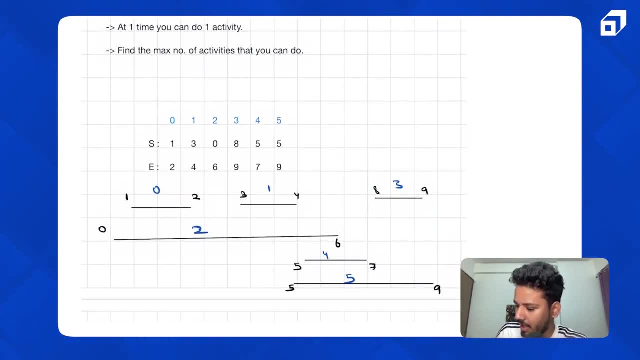 First activity starts at time 3 and set time 4. Second activity starts at time 0 and set time 6. So on and so forth. So, just to make this easy, what I have done is I have drawn these activities. 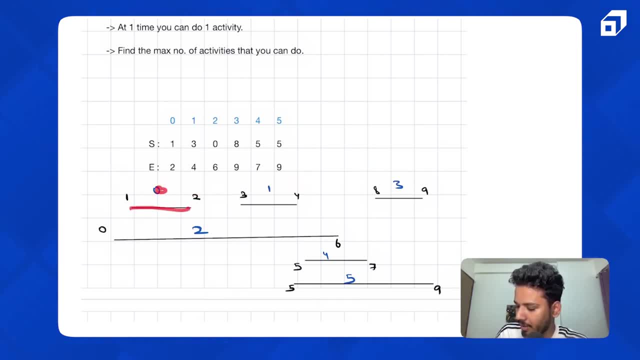 As the number line. So 0th activity happening in 1 to 2.. First activity happening in 3 to 4. Then second activity happening 0 to 6. So on and so forth. Let me change the page style. 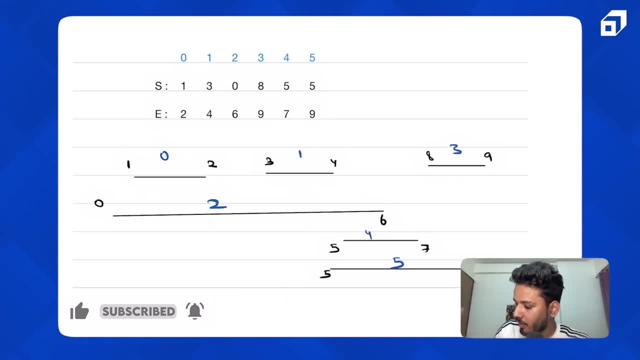 So maybe we can have just normal lines. First of all, let's try to see what is the solution. So what all activities, maximum activities that I can do? So I think I can do 0th activity, Then I can do first activity. 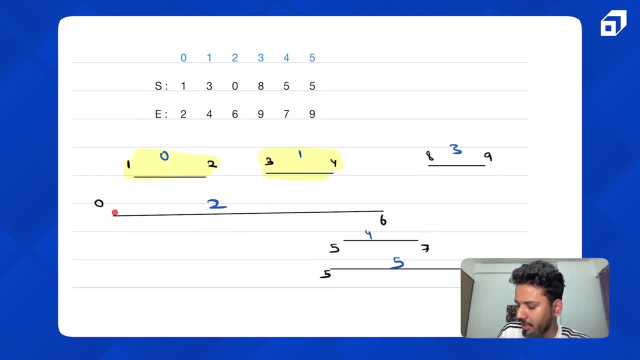 Now I cannot pick second activity right, I mean, and initially I did not choose this one, Because then, instead of this, because instead of this I can do 2 activities, Then, just because I have this, I think just to make the diagram beautiful, they both are starting at 5.. 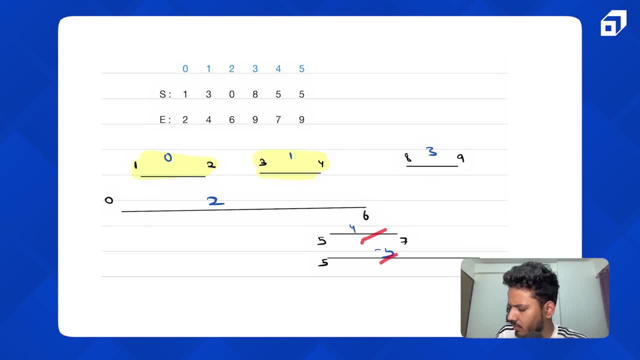 Now this is ending at 4.. So I think I can pick any of these 2.. So let's do one thing. Let's pick which activity. If I pick this activity, Let's correct the numbering 5 to 9.. 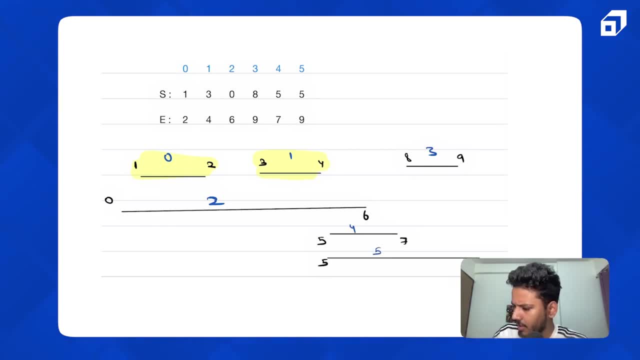 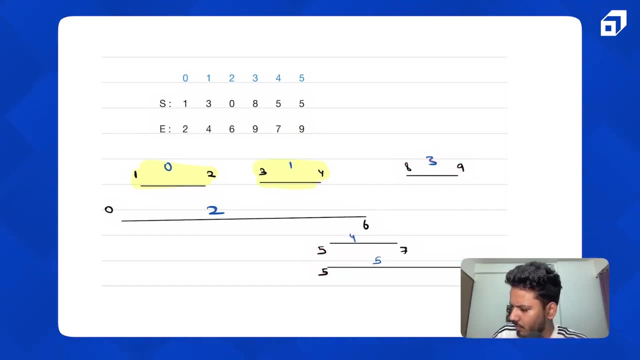 It is 5th activity, So if I choose this activity, I would be able to do only this one. Instead, let's do these 2 activities. So what we can do is we can do these 2 activities. 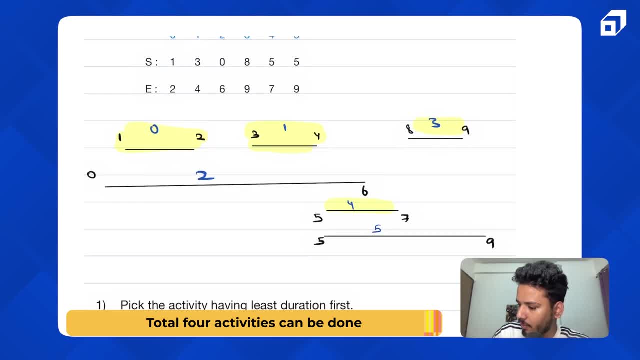 So total? I think answer is 4.. So total 4 activities can be done for this scenario, right? Total 4 activities we can do. These are the 4 activities. Whatever you do, whatever order you pick, you cannot do more than 4 activities. 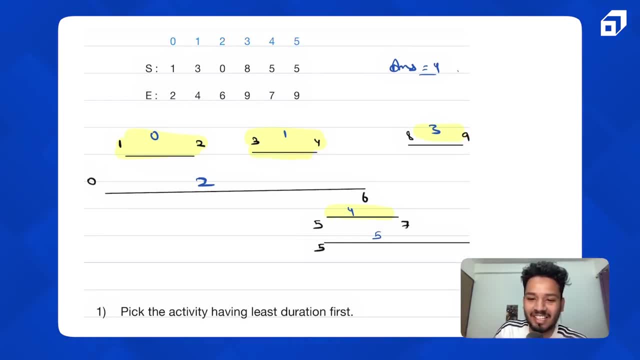 Now, when we see this question- And I initially mentioned it, It's a greedy question. Without even that, What is the first thing that comes to our mind is: Let's try to do what We will take our approach. We will pick the activity having least duration first. 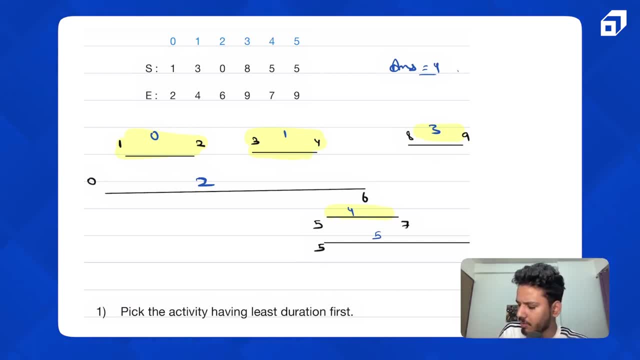 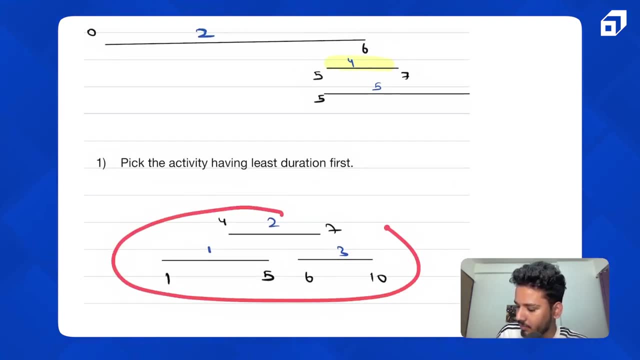 Sounds like a plan: Pick the activity having least duration first, So shortest activity You complete first, Then so on and so forth. So I have an example for that In this one. This is first activity, Second activity. 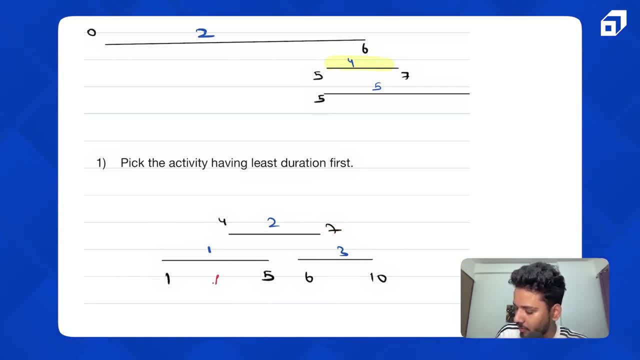 Third activity. This is taking 4 units of time: 4 units of time And 3 units of time. So what are you going to do? If you keep this approach, That you will pick activity with least duration, You will pick this activity. 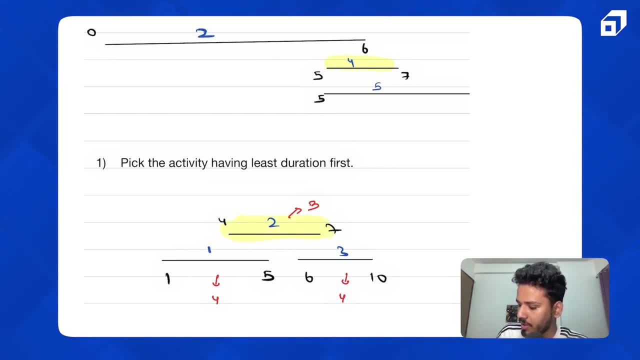 So let's say we pick this activity. Now what's the problem with picking this? I cannot pick first and third activity, But is the answer really 1?? Can you do only 1 activity? No Right, You can do these 2 activities. 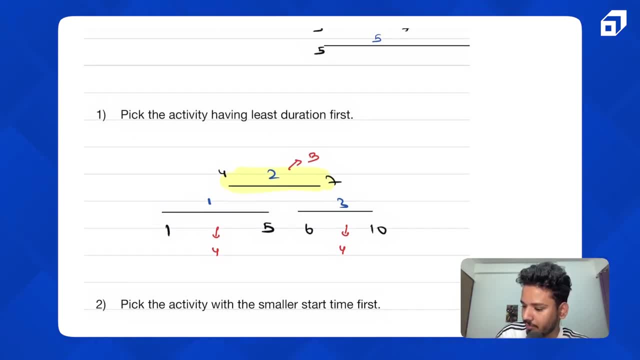 So this approach is wrong. So this approach of choosing activity with least duration fails What else we can do. So let's move on to the next idea We might get: Pick the activity with the smallest start time first, So activity which is starting early. 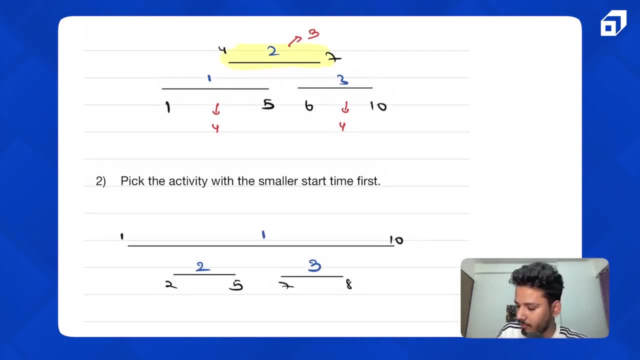 I will pick that up. So let's start. These are the activities. So I will pick this activity First activity first, Because it is starting early, And then I cannot choose these 2.. The other 2 activities: 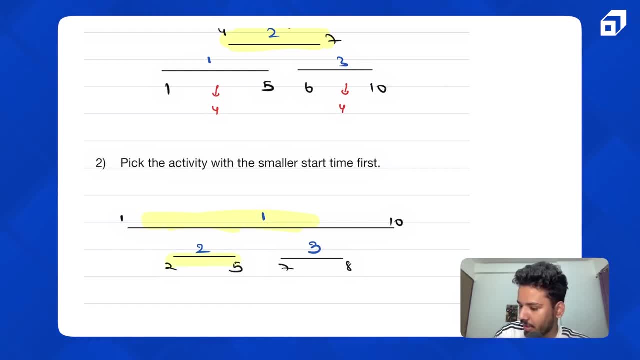 Because they are conflicting with the first activity. Correct, So I can do only 1 activity, But is the answer really 1?? No, Answer is 2.. So this approach also fails. Haha, What else we can do? 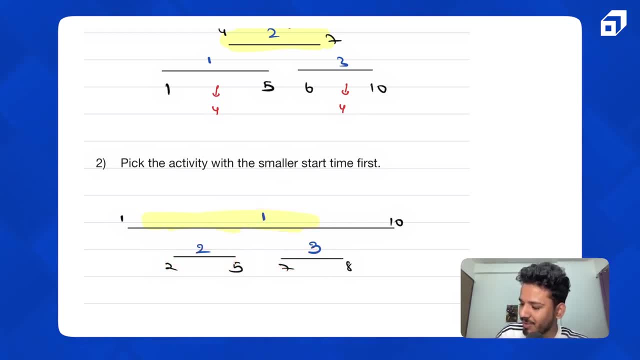 So let's move on to the next idea. We might get Pick the activity with the smallest start time first, So activity which is starting early, Haha, What else? So only 3rd option left. What is the option? 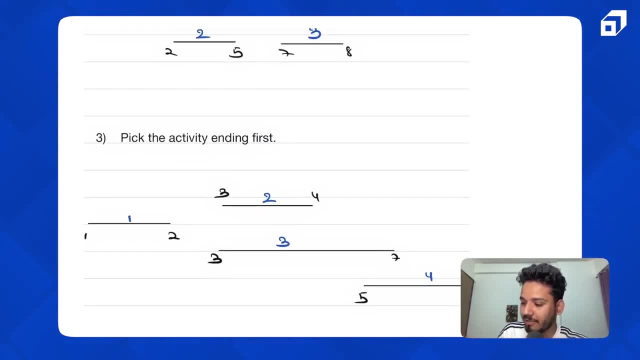 Pick the activity ending first First. Okay, The activity whose end time is short Ending, We will pick that one first. So let's try this approach Again. I am not going to Why this will work or this won't work. 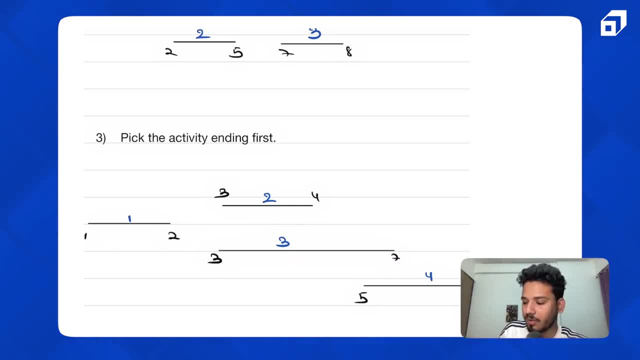 For this idea. Let's just see. So what we will do. We will pick Out of all the activities. This is the activity ending first, So let's pick this one. After this. I have These 3 activities. 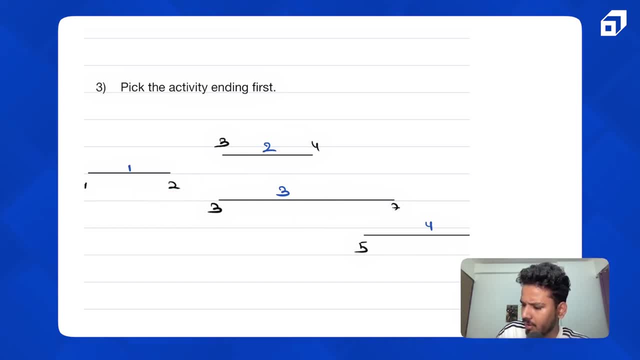 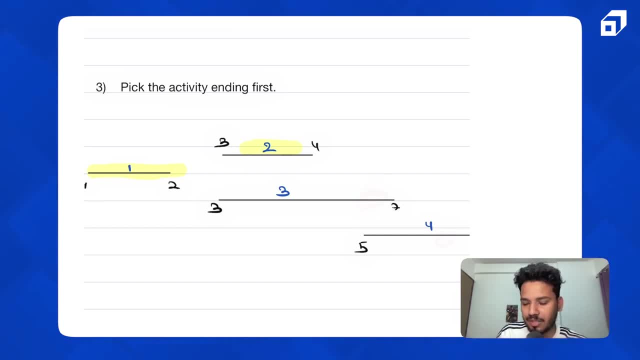 Now, out of these 2 activities, This activity's ending time is first, So this should be picked, But It is already conflicting with my second activity And remember, We can only do 1 activity at time, So this cannot be chosen. 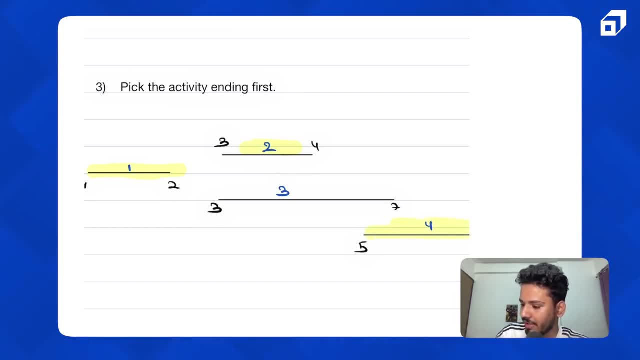 Now this is left. Let's choose this. So we got 3 activities And I think for this one the answer is 3.. So this worked. But will it really work or did I smartly pick the examples? 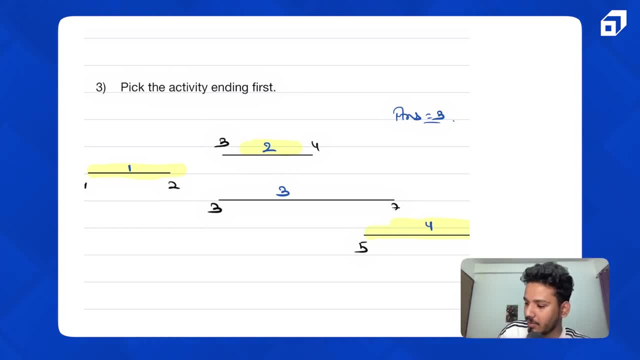 an example in which this is working. so, actually, this will work. this greedy idea will work, and the reasoning behind that is: you pick an activity which is ending first so that in your time zone, you will have more time left to complete pending activities, right, which was not the case when you. 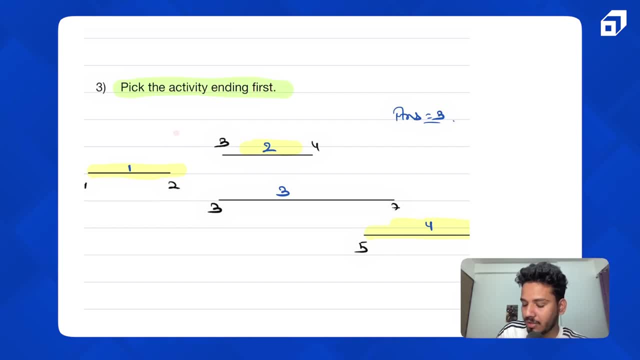 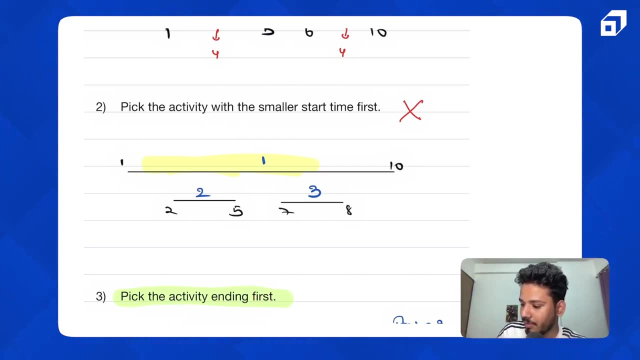 pick the activity with starting time first, that doesn't mean it was ending first. also, right, when you pick an activity which is starting early, that doesn't mean it will end early also. for example, you have- you saw this- that it was starting early, but it was it was ending, uh, at the end or most. 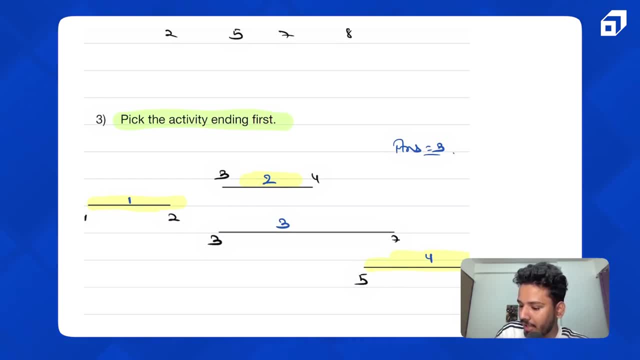 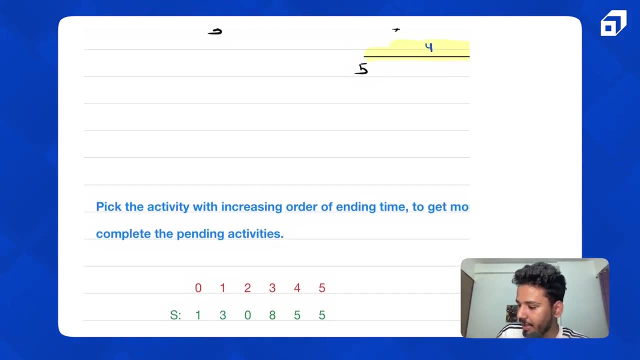 late. instead, if i pick an activity which is ending first, i will have more time left to complete more activities. right, and which is what i want. so the idea is: pick the activity with increasing order of ending time. so means what the activity which is ending first, pick it first to get more time. 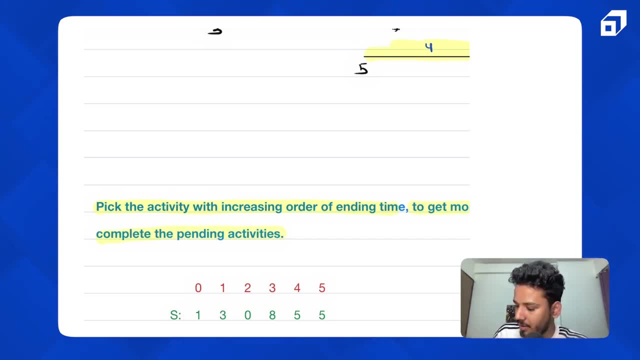 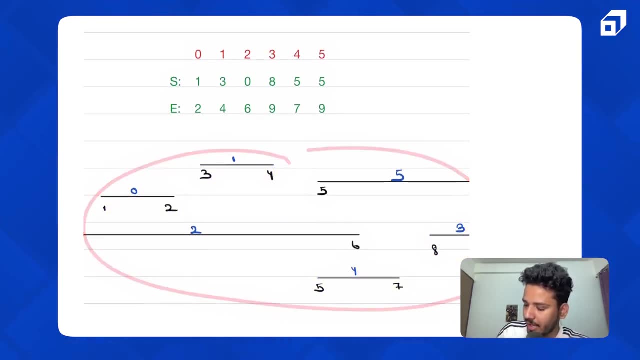 to complete the pending activities. so let's just see, let's just try to do it for this one. so these are the activities, and i have drawn them on number line. so what will i do? i will pick the activity ending first. so this is the activity which will. 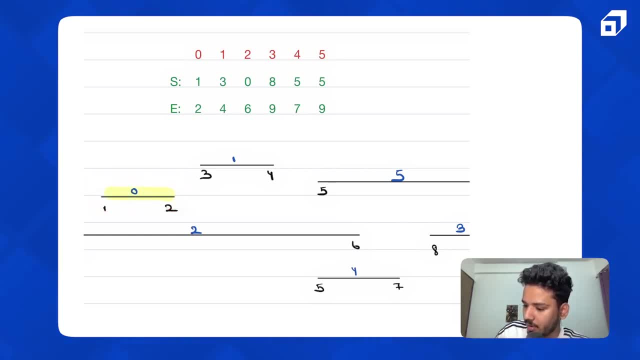 get picked first, so we can do this. now. what next? this activity has the next smallest ending time, so let's pick this one then. this activity has the next earliest ending time, but it is conflicting from my activities which i already did, so i cannot choose this one. now what next? 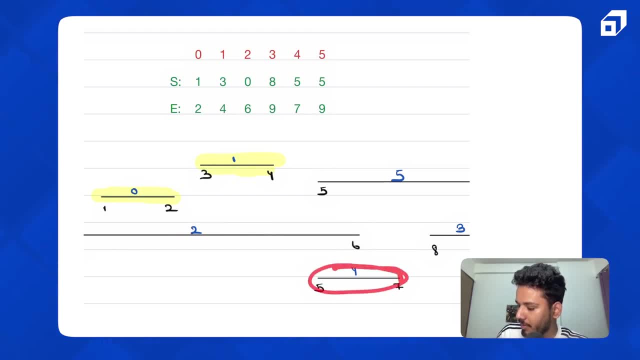 this activity. this activity has smallest ending time after this one, so let's pick this one. what next? both these activities are ending at the same time, but this i cannot choose right, because this is already conflicting with one of the activities that i have chosen, so i will pick this activity. 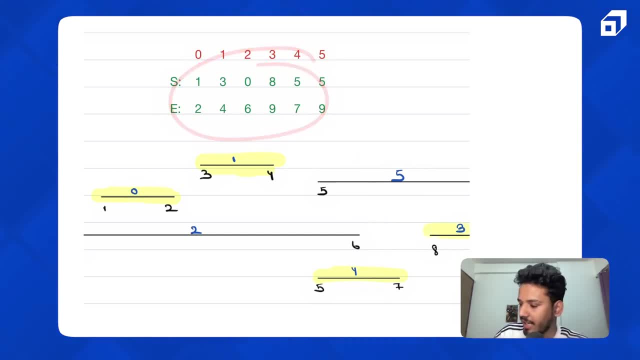 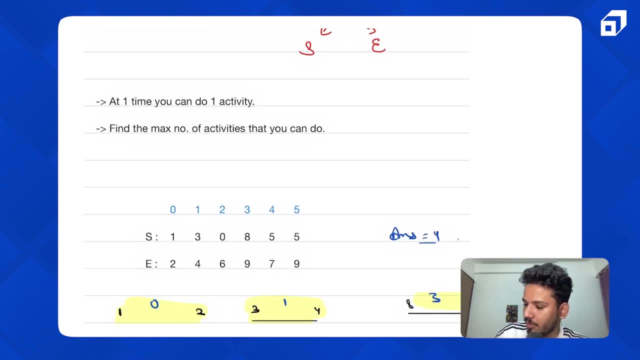 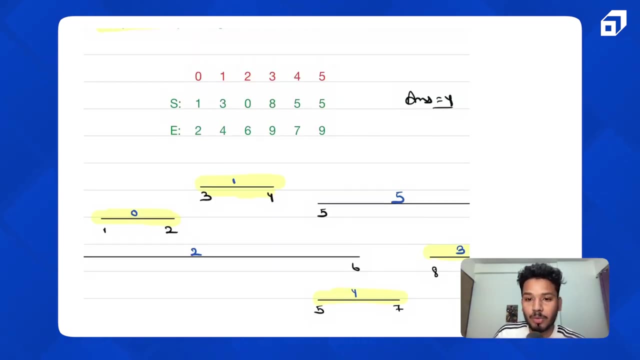 so for this array, this start and end time, this set of activities, i can do total four activities, which is my answer, and this was the initial example. so you saw this. is it four activities you can do? again? the answer is: reasoning is very simple. you pick an activity ending first because that will give you more time. 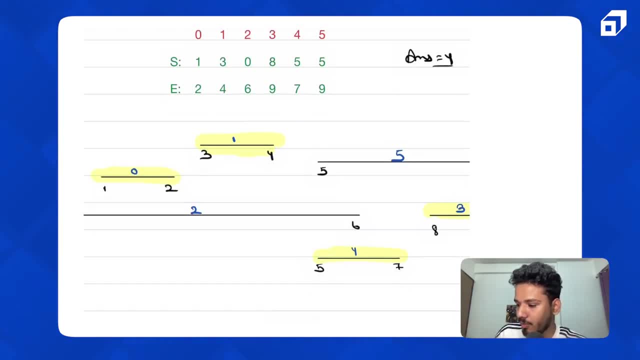 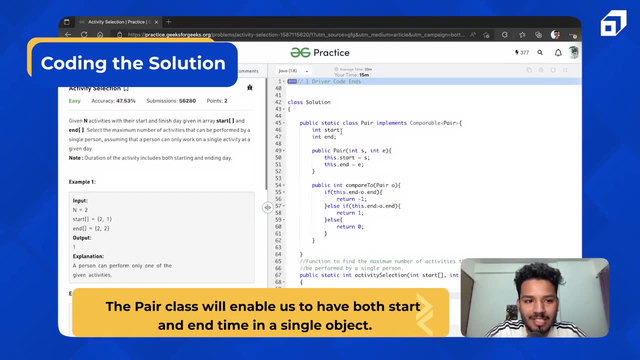 so to complete all the pending activities, now let's move towards the code part. first of all, i need a pair class. why i need a pair class? because i want my start and end time to be clubbed together and whenever i mean, basically i can sort the end area, right, i am. 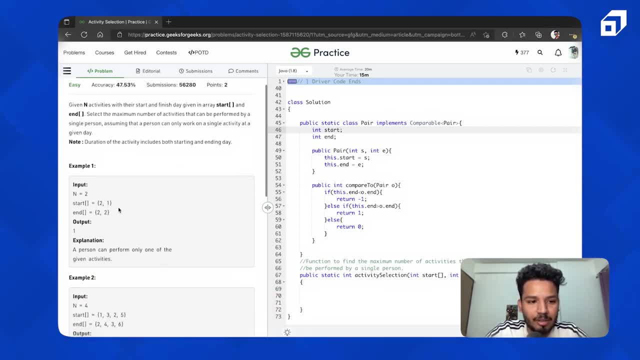 given a start array and an end array for start time and end time. if i sort the end array, how would i know that? what is the respective start time of that corresponding end time? so for that i need to make a pair out of them. so for that i have created a pair class, very simple. now then. 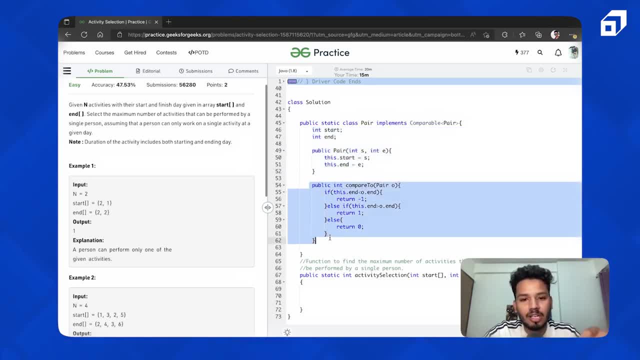 this is just a comparator, custom comparator i have implemented. why? so that i can get- uh, i can sort the pairs. now i don't have to sort an area. i need to sort pairs. i want the smallest pair, i mean the pair with earliest end time and, corresponding to that, a start time. 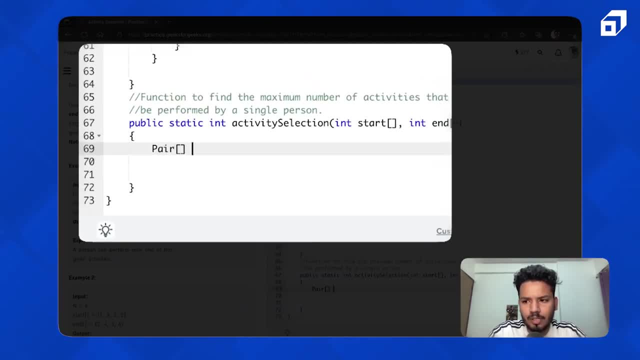 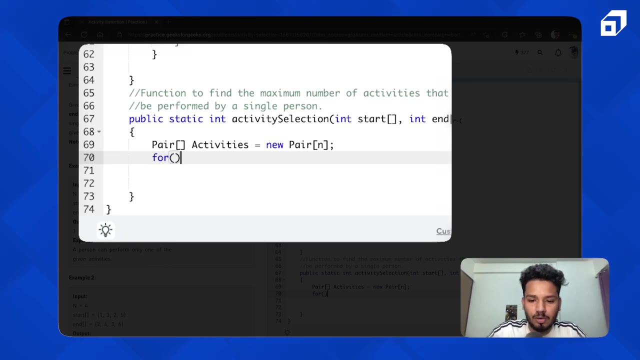 so let's create an array of pairs. pair array- let's call it activities- and then is equal to new pair of size n. and then what? so i've created a pair array for all the activity i'm going to store. now let's store them, for: n i is equal to 0. i is less than n i plus plus. so activities of 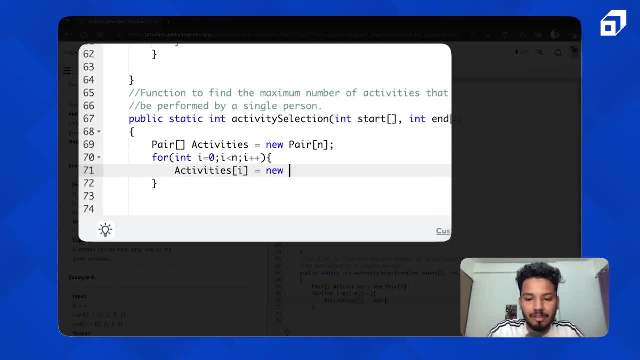 i for every activity i need to store, i mean every pair. i need to store new pair and each pair will contain the corresponding for one activity, start and end time. so basically, now i have n pairs, every pair contains start and end time of an activity. now i need to sort them up. so arrays, arrays dot, sort activity. 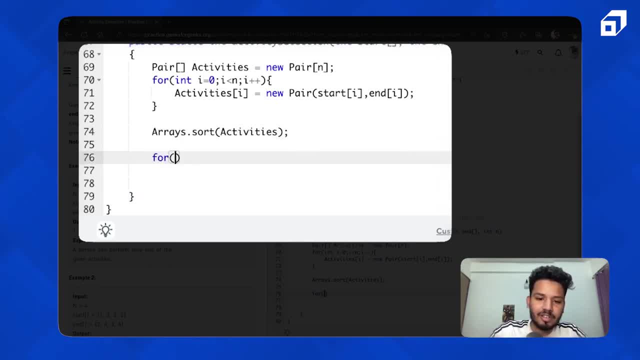 so active. all the activities got sorted, so let's traverse over the array now. in the array i have all the pairs stored and the pair with smallest end time will come first. so for and i is equal to 0, i is less than n, i plus plus. and then what else do i need? i need answer variable to store the. 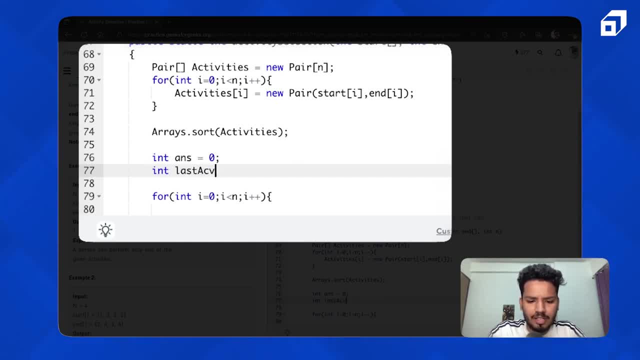 final answer and it and last activity. and when did the last activity end so i can decide whether the new upcoming activity i can choose or not? because, let's say, your last activity ended at time 6 and new activity, which has a later end time, uh, let's say at 9, but has a early start time. 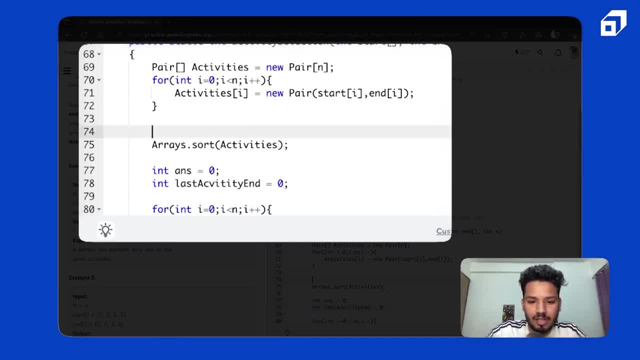 you cannot pick that right. if your current activity ended at 6 and the new activity which ends at 9, obviously the new activity will have a later on end time. but let's say it start was at 3.. you cannot pick that right. you have to make sure your new activity start time is at least greater than. 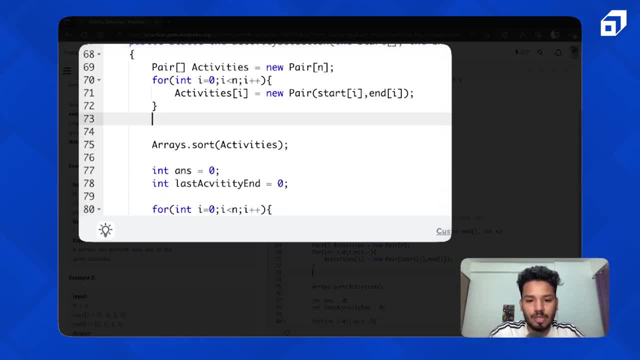 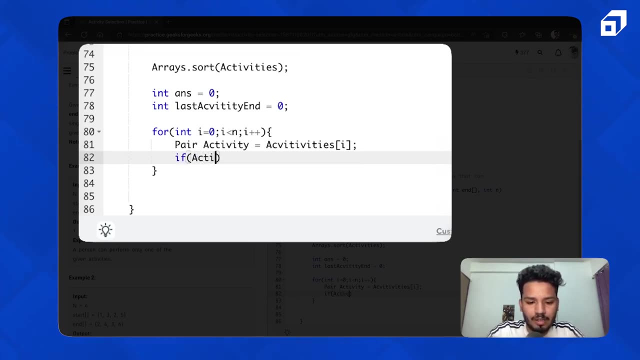 the last activities and time which you picked. so then, pretty simple, i will traverse over the array. now let's get the activities one by one. pair activity is equal to t with t's of i. and then what if? if it is the certain line type we're going to pick, Alright. the activity ended at 9. 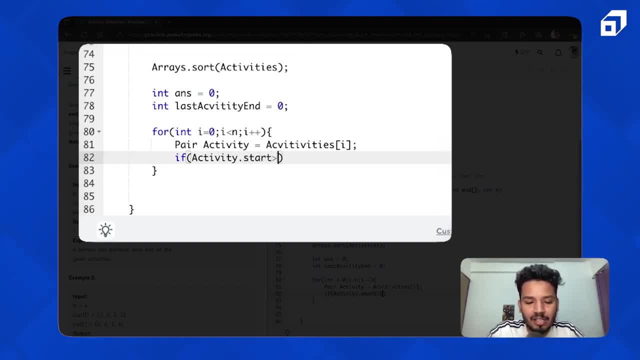 so, for instance, that is the last activity we didn't pick was obviously t and group directory. we have seen it there, but let's say so i will pick this two and think that i can say that this will be the end time. then last activity time must be greater than X. it has to be greater than. dot actual activity that you have dot start time. it has to be greater than last activity end it last activity end time. then only i can choose it. so, and now the last activity and one last period, and will become the new activity that you have picked. it's end time and your answer will become plus. now in some of the portals you will get it said greater than equal to n and the result: this will give a place to set greater than equal to 0. 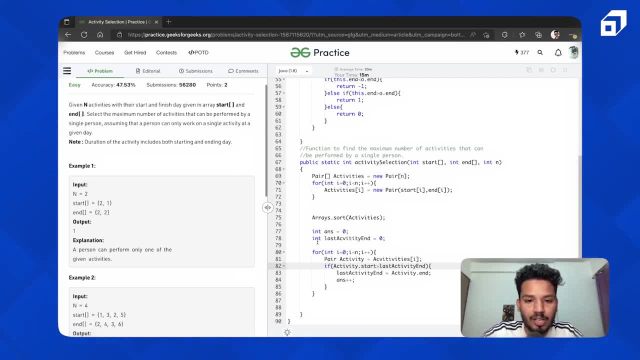 here it's only greater than because, uh, they say, when current activity ended at two, you cannot start a new activity at two, you have to start it at three. that is why i'm picking greater than okay and then finally i can return answer: hope. everything is fine. then maybe let's compile.